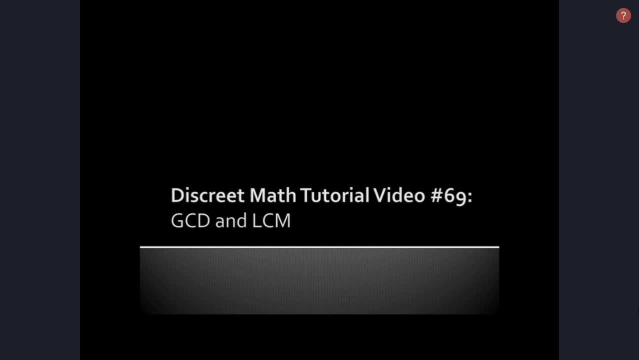 LCM, GCD. Just so you know, GCD stands for two meanings: Greatest Common Denominator and Greatest Common Divisor, While some books may state that the Greatest Common Divisor is also known as Greatest Common Factor, Highest Common Factor, Greatest Common Measure or Highest Common Divisor. Anyhow, same point. 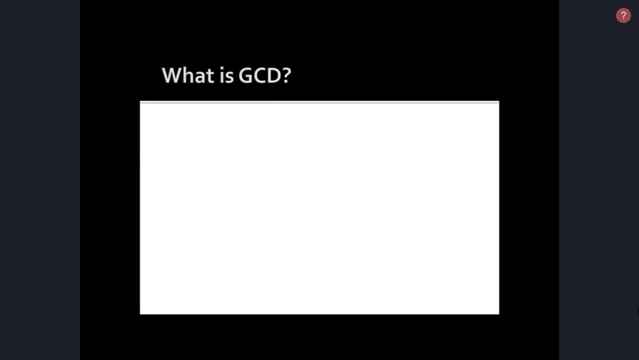 It comes down to this question: What is GCD? In mathematics, the greatest common divisor of two or more integers, which are not all zero, is the largest positive integer that divides each of the integers. For example, the GCD of 8 and 12 is 4.. Before moving forward, don't mistaken GCD as LCM. 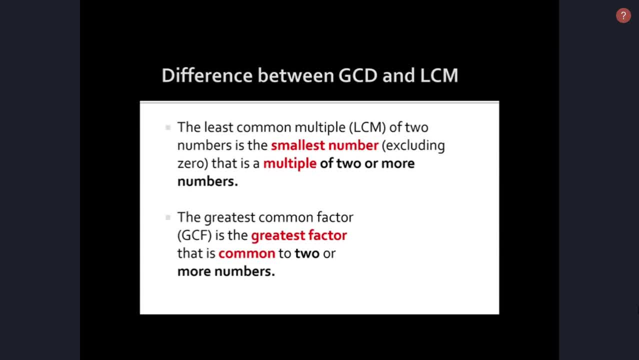 GCD is usually mistaken for another mathematical term. Again, don't mistaken GCD as LCM. The least common multiple or LCM of two numbers is the smallest number excluding zero. that is, a multiple of two or more numbers, The greatest common. 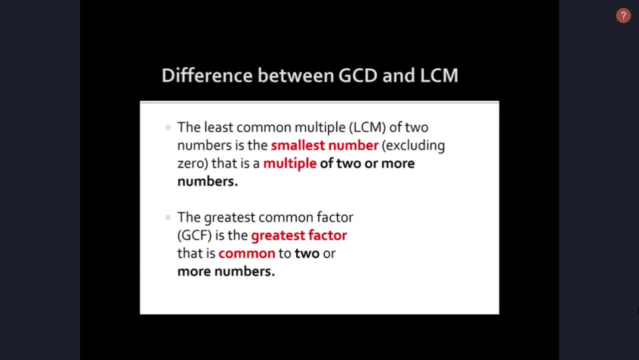 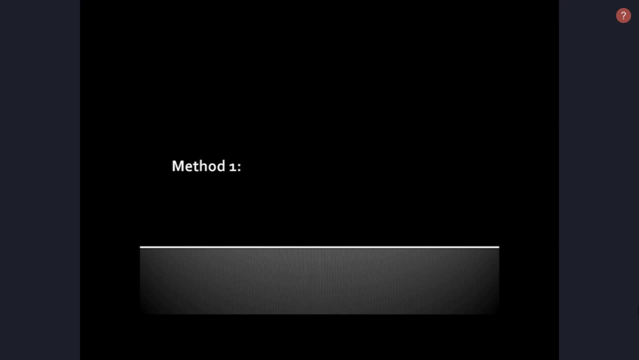 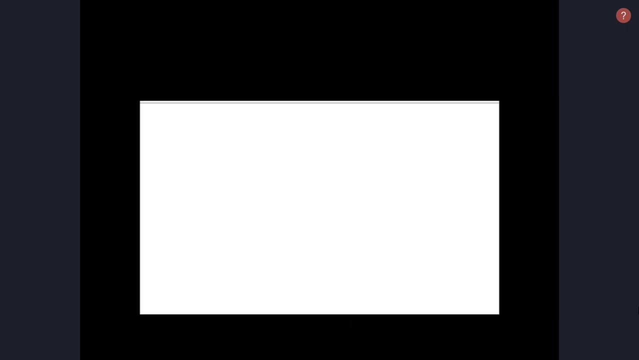 factor, or GCF or GCD, is the greatest factor that is common to two or more numbers. How do we find out and get the GCD for two integers? Well, there are four methods. The easiest one would be by listing all the divisors of the given numbers. 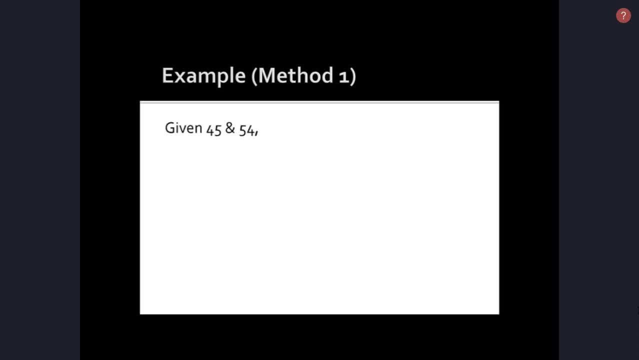 As an example for method 1, let's set it to be 45 and 54.. List all the divisors or any number that divides the number, which would not come up to any remainder. As for 45,, we got 1,, 3,, 4,, 5,, 6,, 7,, 8, 9,, 10,, 11,, 12,, 13,, 14,, 15,, 16,, 17,, 18,, 19,, 20,, 21,, 22,, 23,, 23,, 24,. 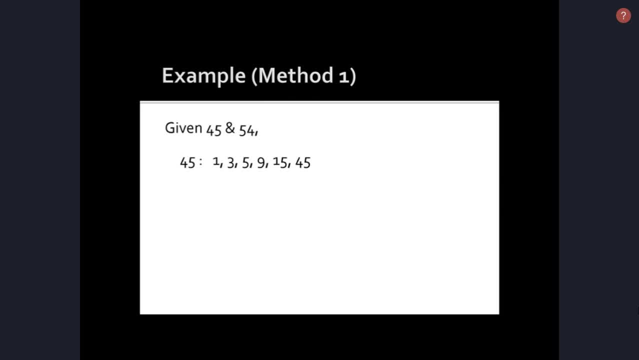 25,, 9,, 15, and 45.. For 54,, 1,, 2,, 3,, 6,, 9,, 18,, 27, and 54. The greatest common divisor for both numbers is 9.. Second method is called prime factorization method. 1,, 2,, 3,, 6,, 9,, 18,, 27, and 54. The greatest common divisor for both numbers is 9.. The second method is called prime factorization method. 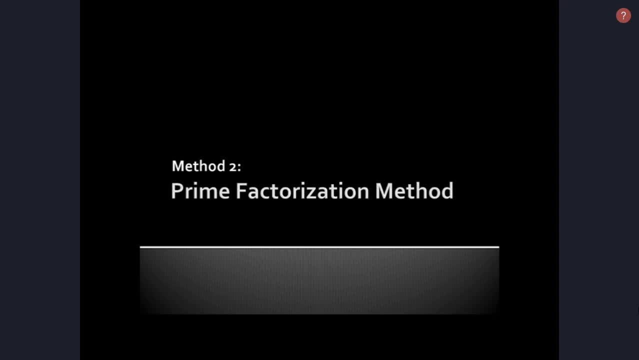 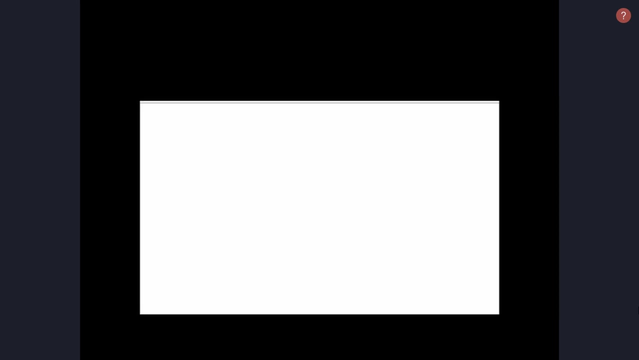 Using this method, first find the prime factorization of each number. The GCD of all numbers is the product of the common prime factors. As an example for method 2, let's set the numbers to be 24 and 60. Continue on getting their prime factors For 24,. 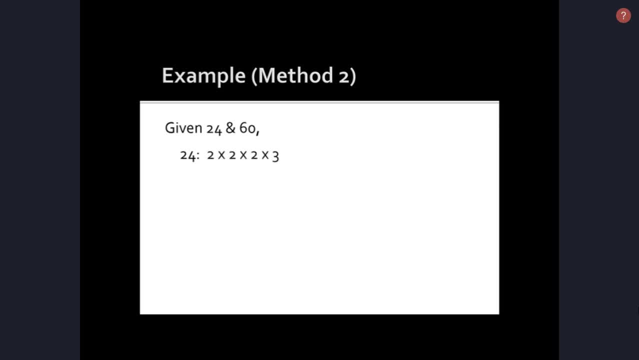 It's prime factors are 2,, 2,, 2, and 3.. For 60.. It's prime factors are 2,, 2,, 3, and 5.. The common prime factors are 2,, 2, and 3.. 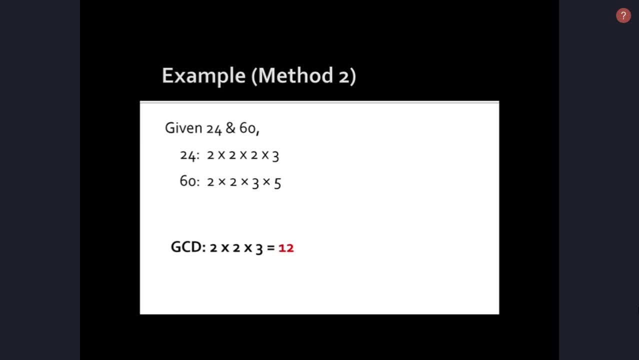 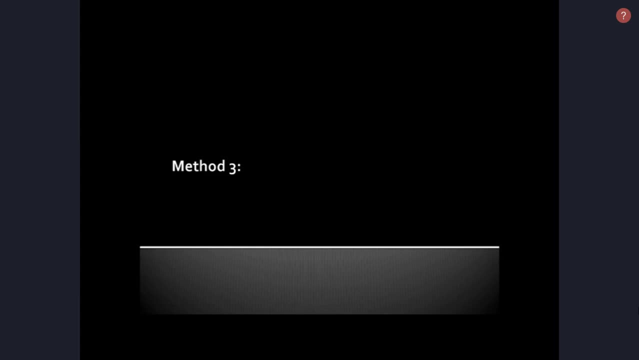 The greatest common divisor of 24 and 60 is the product of this common prime factors. As for the given, 2 times 2 times 3 equals 12.. Third method is division by primes, As what the method suggests divide the numbers by their common prime factor. 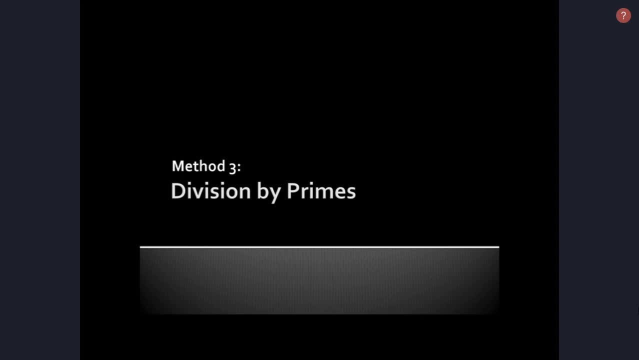 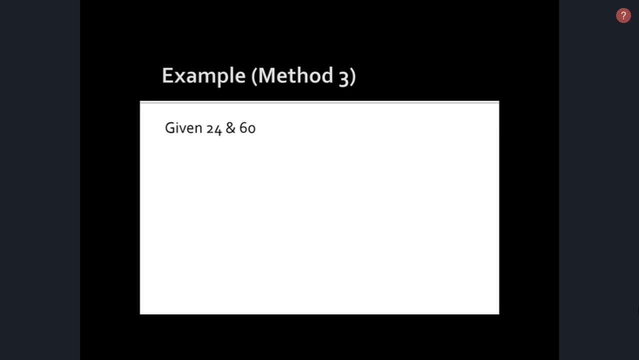 You just have to do it multiple times. Easy as that. Stop when you no longer can come up with a common prime factor. As an example for method 3, let's set the numbers to be 24 and 60. First, divide all the numbers by the smallest prime factor that can divide both of the numbers. 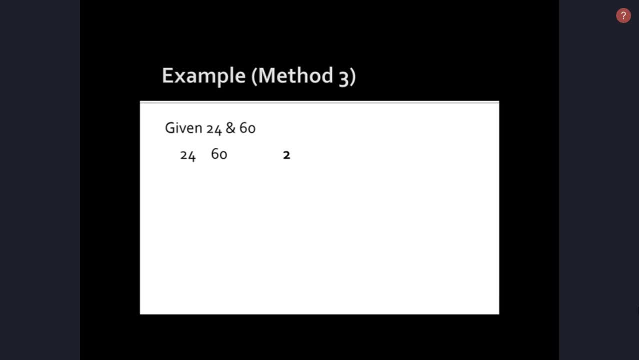 The smallest prime number that divides 24 or 60 that I could be thinking of is 2.. Continue the steps until we can find any prime numbers. There is a number that can divide all the numbers on the right side. The GCD is 2 times 2 times 3 times 1, which is equal to 12.. 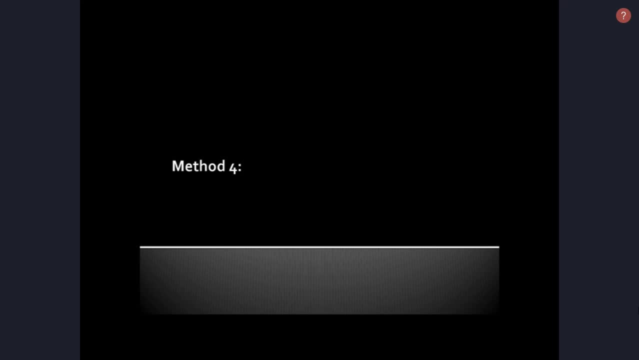 The fourth and final known method is called the Euclidean. This is known as the Euclidean algorithm According to its method name. the algorithm was as proposed by one of the ancient mathematicians, Euclid. This algorithm finds GCD by performing repeated division starting from the two numbers we want to find the GCD of, until we get a remainder of 0. 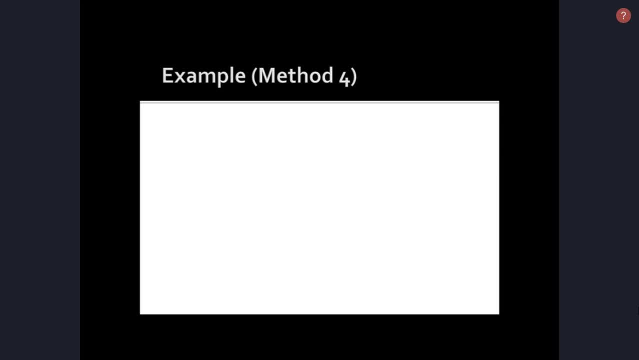 As an example for method 3, let's set the numbers to be 24 and 60. that can divide both of the numbers. for method 4, let's set the numbers to be 24 and 60. Divide the larger number by. 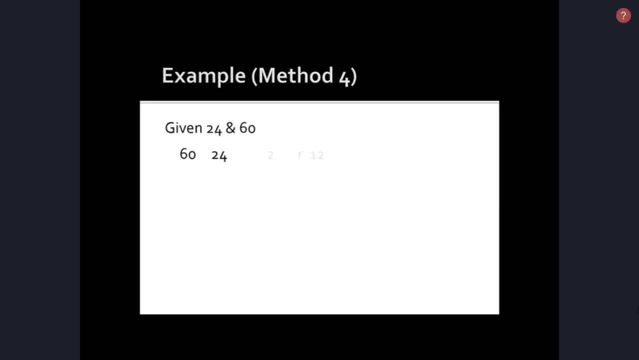 the smaller number. Next is we must divide the smaller number from the previous equation by the remainder from the last division. Repeat until you get a remainder of 0.. The GCD is the smaller number from the previous equation before you came up with the remainder of 0,, which is 12.. Therefore, the GCD is 12.. 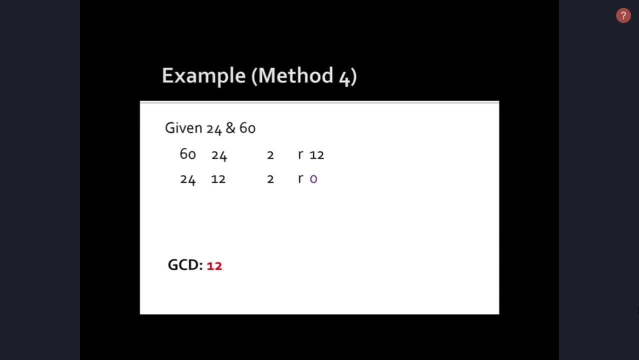 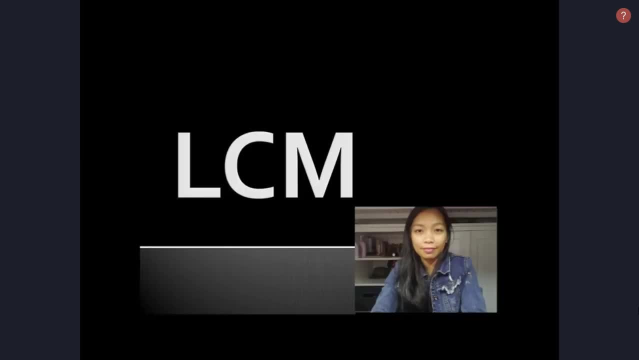 The latter part of this tutorial video is regarding these common multiple. Again, what is LCM? The least common multiple or LCM of two numbers is the smallest number excluding 0, that is, a multiple of two or more numbers. Digging: 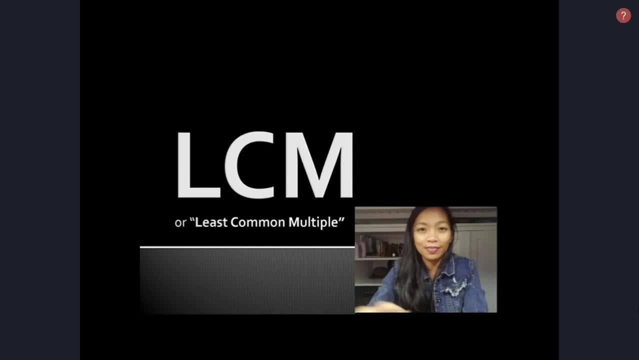 into the concept. there are three known methods on getting the LCM. The first one is the LCM. The second one is the LCM. The third one is the LCM. The fourth one is the LCM. The fifth one is the LCM. The sixth one is the LCM. The sixth one is the LCM. 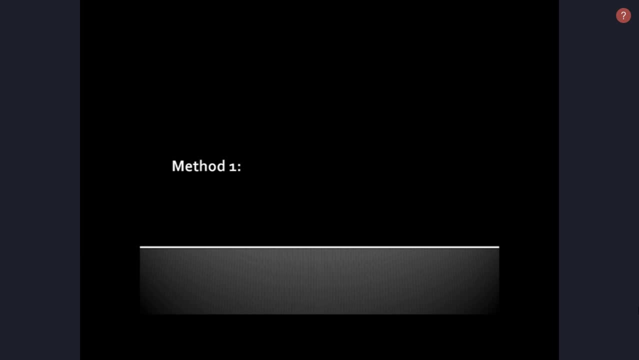 The first method is called prime factorization method. Using this method, first find the prime factorization of each number. In contrary with GCD, the factors are written in index form and the LCM is the product of each prime factors with the greatest power. 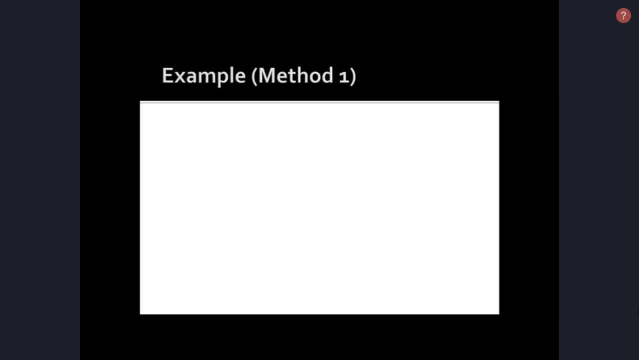 For method 1, let's set the numbers to be 24 and 60.. Write the prime numbers in index form: For 24,, we have 2 times 2 times 2 times 3, or 2 cubed times 3.. For 60, we 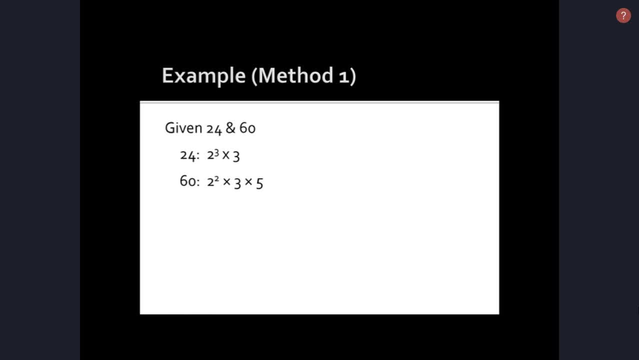 have 2 times 2 times 3 times 5, or 2 squared times 3 times 5.. The least common multiple is the product of each prime factor with the greatest power. So for the above example, the LCM is 2 cubed times 3 times 5 is 120.. 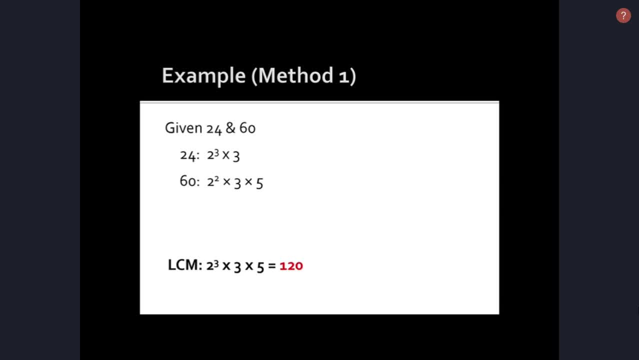 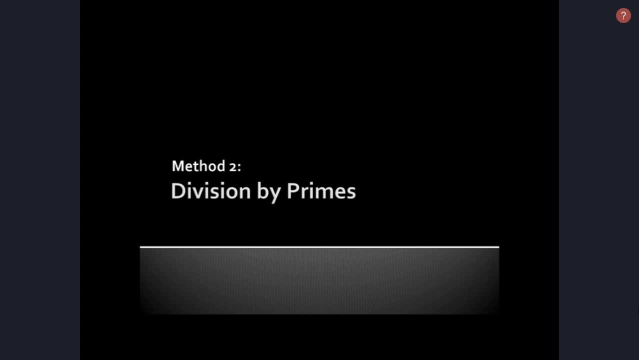 For the second method. it is called division by primes, As what the method suggests divide the numbers by their common prime factor. You just have to do it multiple times Easy as that. Stop when you no longer come up with the common prime factors. 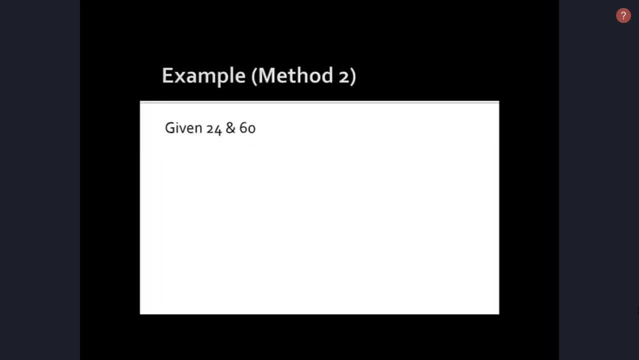 As an example for method 2, let's set the numbers to be 24 and 60 again. First, divide all the numbers by the smallest prime factor that can divide both of the numbers. The smallest prime that divides 24 or 60 is 2.. Continue the steps to.